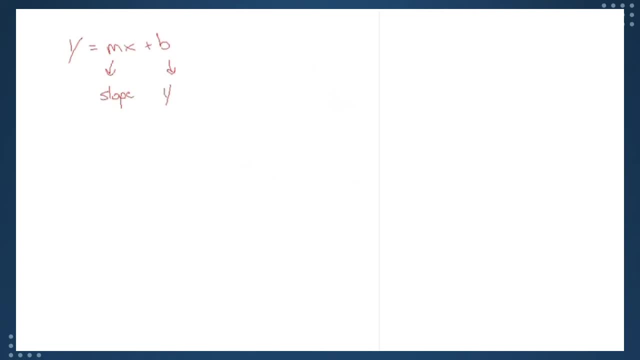 And b being the y-intercept. So the first part of today I want to talk about how they can kind of strategically test you on these things. Sometimes it's really easy, Sometimes it's really hard. So we'll kind of work our way up in the questions we're doing. But I 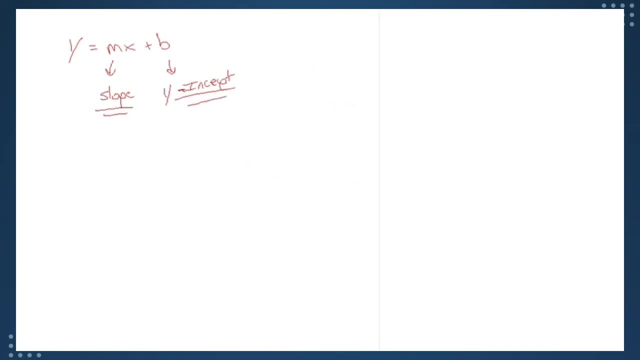 do feel confident that by the end of today everyone should be looking at coordinate geometry, kind of in an algebraic sense, Which I think is a really cool way to think about these things. So first question I'm going to put up for all of you who have been here before and you know: Answer the question. 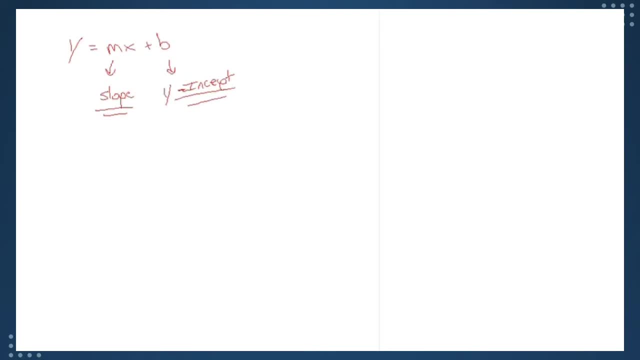 Put your answer in the chat box, We'll go to the solution And, of course, we'll do more. So first question is this here: Remember everyone: just make sure you're muted. I think when you get accepted into the meeting you're unmuted. So if you're not muted, you're muted. 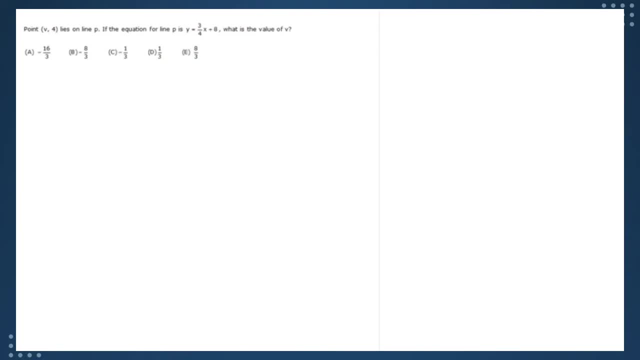 So if you're not muted, you're muted. So if you're not muted, you're muted. So if you're unmuted, you're unmuted. So maybe something you have to manually do on your own: you, you, you, you. okay, that's about two minutes and I presume that that wasn't all that bad. 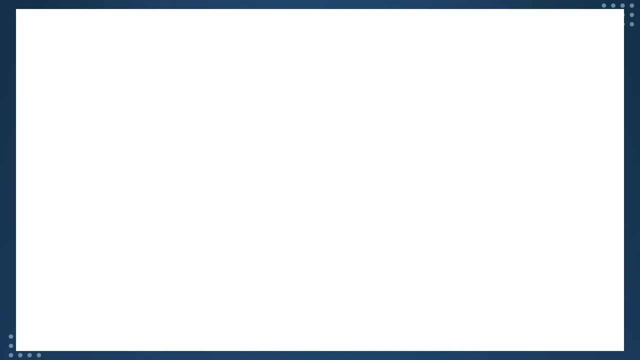 for everyone. so the interesting thing about this question here is they're giving us a coordinate, set of coordinates, where we have V being the x-coordinate or being the y-coordinate. so, in essence, what they're doing here is they're testing us on our ability to know. 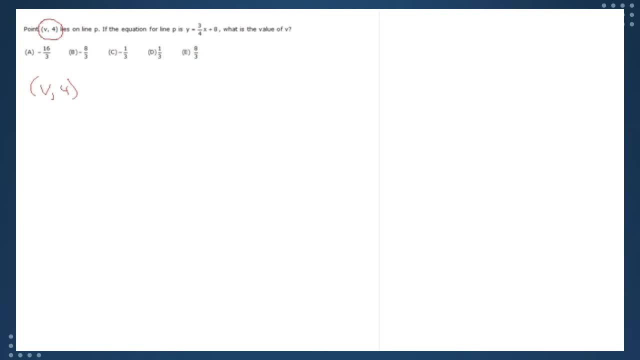 that V can replace the X and that 4 can replace the Y. so we have 4 equals 3 fourths V plus 8. and we're just going to do the math. we bring the 8 over to the left. that becomes minus. 4 equals 3 fourths V, minus sure how that happened. 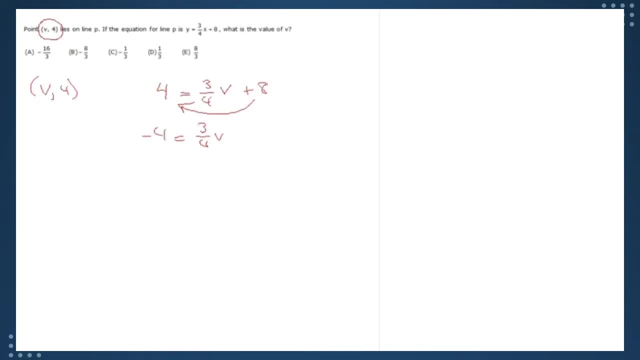 a lot of getting me word back. okay, minus 4 equals 3, fourths V. we bring the 4 over. negative 16 equals 3, V divide both sides. that's our answer. so this is a very kind of basic version of what I'm about to show you, which is a question where we have more plugging. but 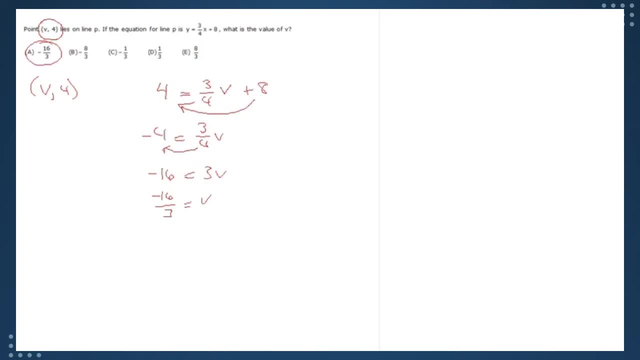 certainly we're dealing with algebra and you know, in the in the same time sense. here the question is: how can we make it more easy? so I want to give everyone a few minutes to try this question here and any question like this. it's interesting. I do this with students a lot. there's definitely multiple ways to get an. 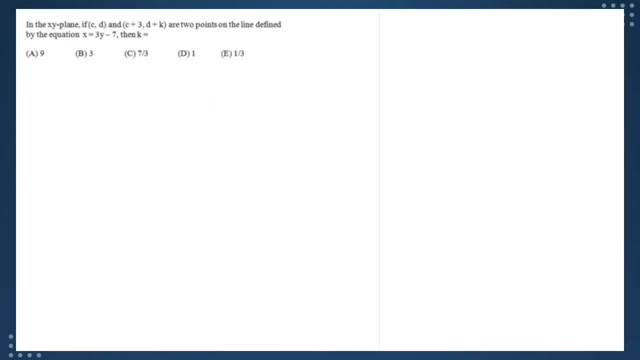 answer with this particular question that I just put up. but you will, I'm going to show you kind of my way of doing it. another said I said in the past, it's okay if you're doing things in a slightly different manner, but this here should trigger the thought of doing algebra. so again, two minutes and a half. 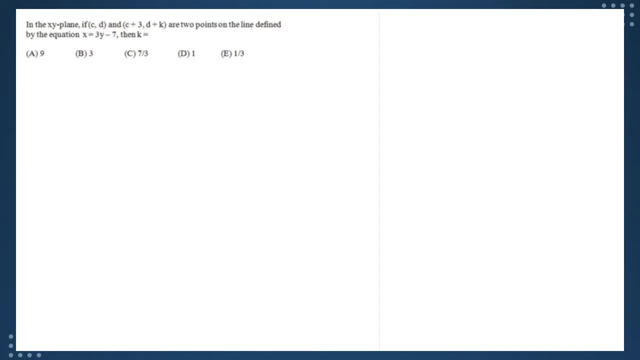 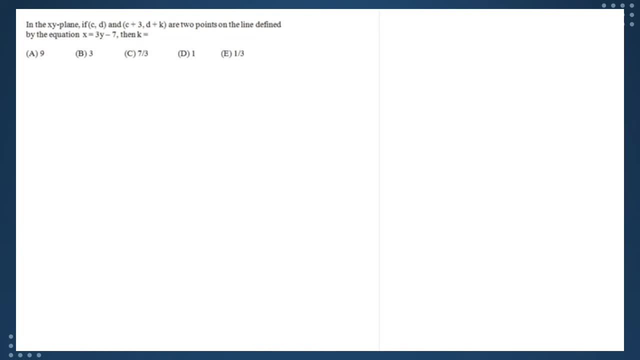 So when I say more elements, what I mean is the fact that you know, we have two sets of points. We have a CD and then a C plus 3 and a D plus K, where C represents the X point, the X coordinate, D represents the Y, C plus 3, the X and D plus K, the Y. 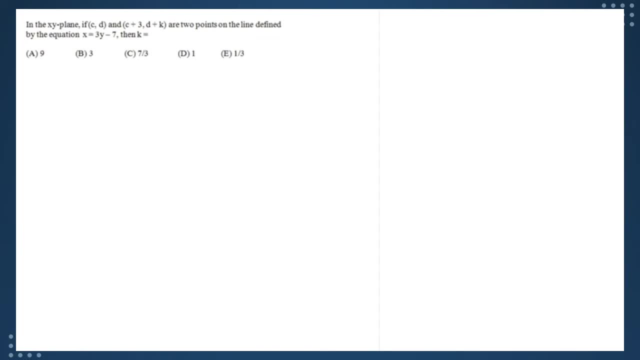 So, effectively, what we're doing here is we're creating two equations with our Cs, our Ds and our K. So the first equation is simply going to be C equals 4.. The second equation is going to be: C plus 3 equals 3 times D plus K minus 7.. 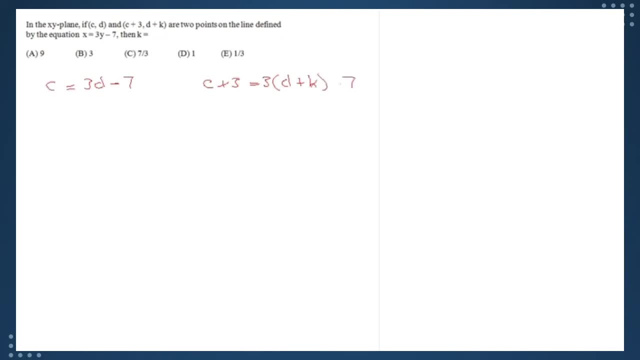 So if we focus in on the right side equation, we get C plus 3 equals 3D plus 3K minus 7.. We bring the 3 over and we say C equals 3D. Now what's interesting here is that they're both equal to C. 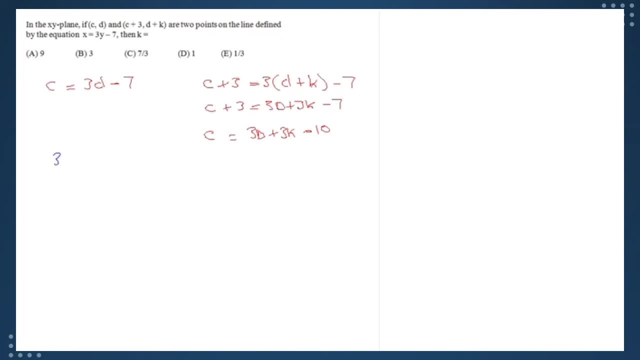 So we can then take them and set them equal to each other. 3D minus 7 equals 3D plus 3K minus 10.. 3Ds- cancel. We have minus 7 equals 3K minus 10.. We bring the 10 over. 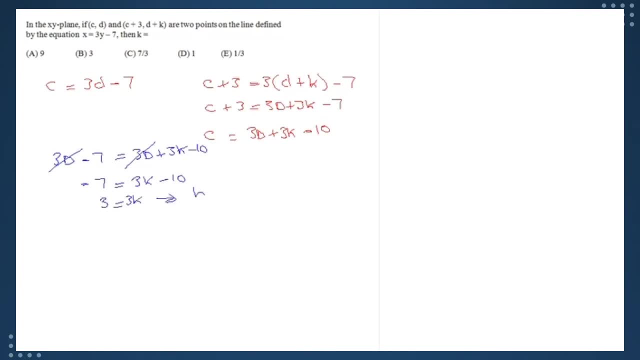 That gives us 3 equals 3K, So of course, K K equals 3K, So that's the circuit of E. So I want everyone to take a good look at this and understand that this is a very important component of coordinate geometry. 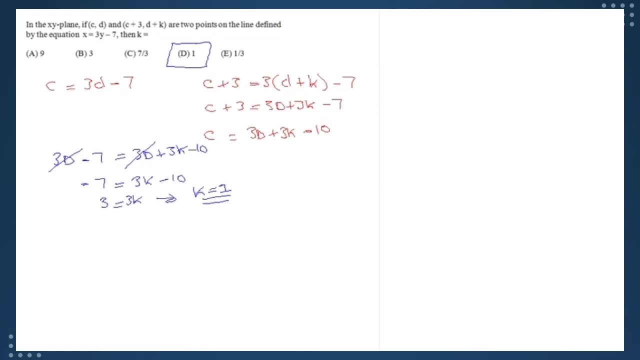 I think one of the things we tend to do when we see coordinate geometry questions is we really default to thinking about this in a way where we're not using algebra? Um, I told you before there are multiple ways to deal with this question. Yes, using the. 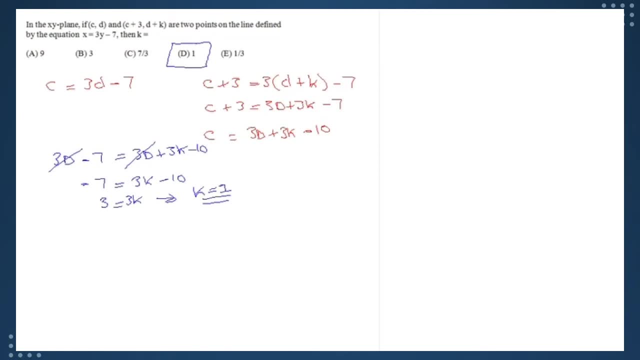 slope formula is one. but my kind of way I think about the GMAT and these exams is that you want to be extremely systematic in your process And for me, if I can set up a line equation and do that, I would do that a thousand times over rather than any other way to deal. 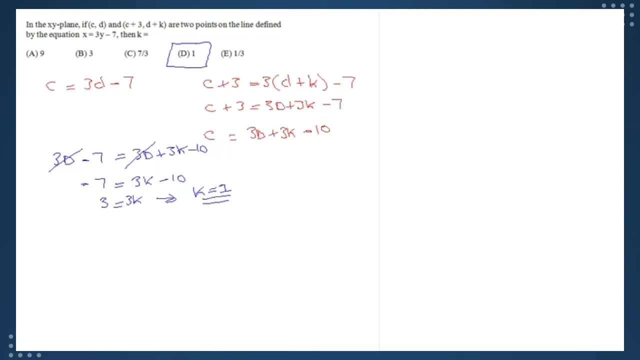 with this question Not to say you can't do other things, and it's not to say that certain things don't feel more comfortable for you, but this is a surefire way you can definitely get this question right. So now I want to get into something that's 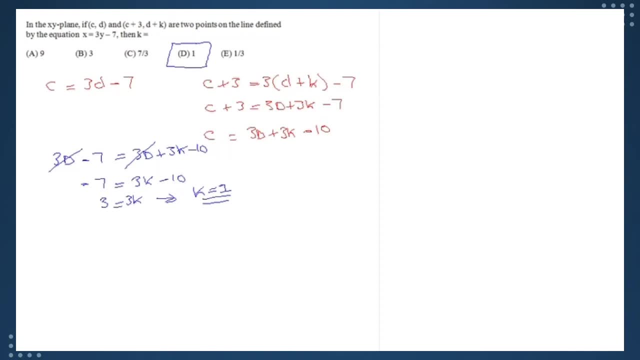 slightly different We're dealing with when you can tell that two of the same points or two points fall on the same line, And when you have the equation of a line, you always have the opportunity to do that. So we're going to do a couple questions. 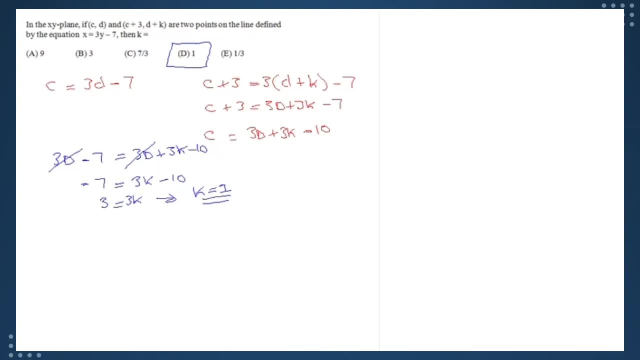 It is similar to what we just did, which you'll see in a second, but it is testing a slightly different component of coordinate geometry. So I'll give everyone a few minutes, then we can kind of discuss this question here. Thank you. 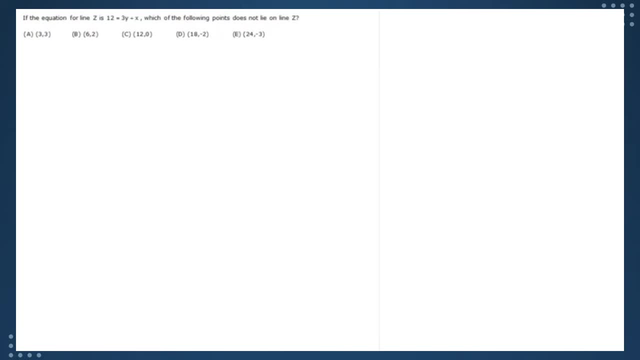 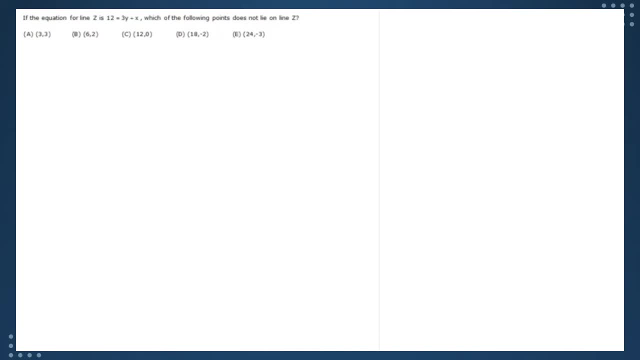 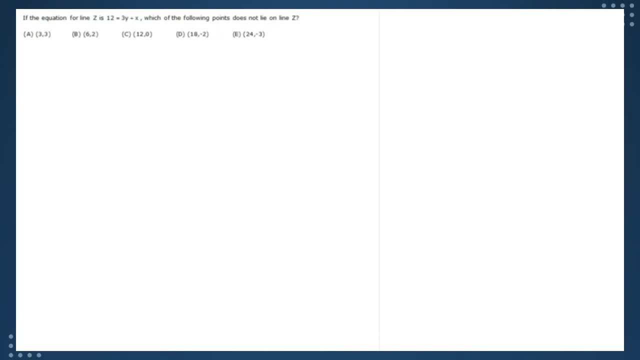 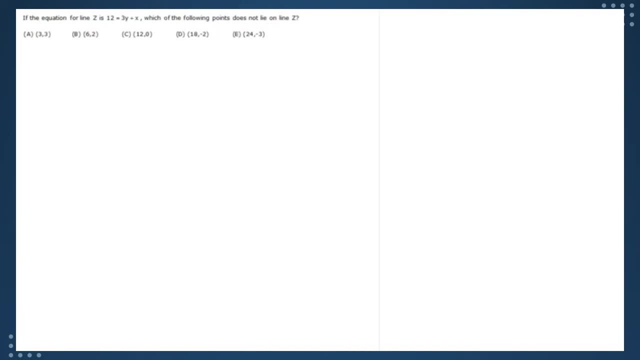 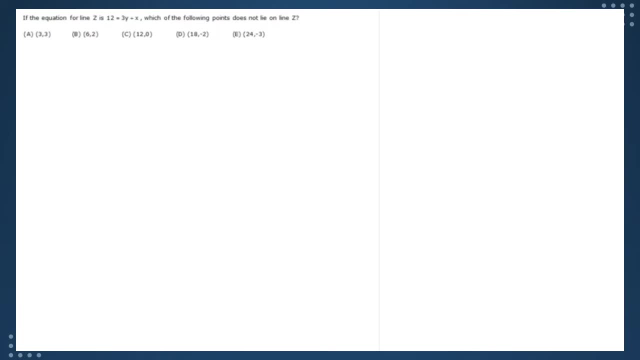 with here right off the bat is the equation of a line. now something again that I like to do. it's not something you have to do, but something I'd like to do- is to get this into the standard form of the line equation. so the way to do that- 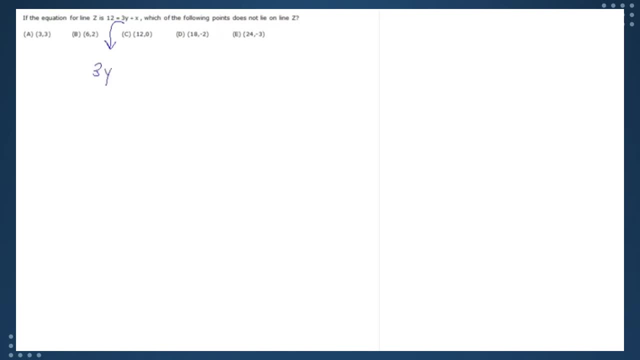 well, first of all I want to set it up so the Y and the X are on the left and I want to isolate the Y. so the first thing is is I bring the X over. point of doing that is to get one step closer to isolating what I believe in: minus X, plus. 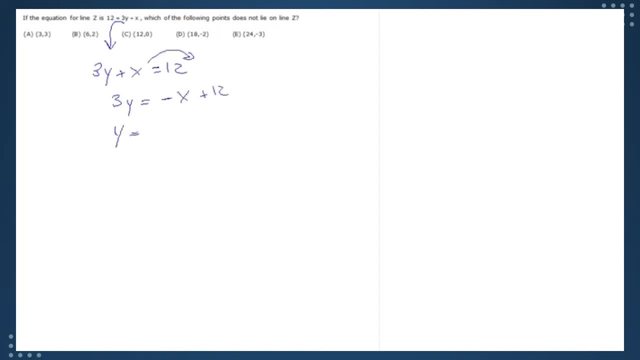 12. Finally, if we divide by three, we get y equals negative one-third x plus four. So the process in a question like this is to then plug in and determine which points will not fall on the line, which means there's going to be one point which will fall on the line. 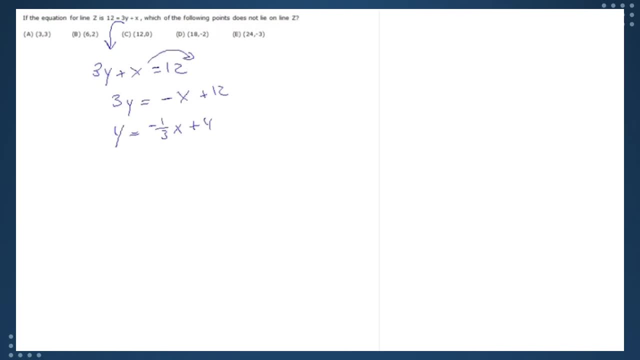 So we can kind of go through our different answer choices and see which one actually does not. So what we have initially here with answer choice A is we have 3, 3. So y is 3, there's an A here and we have negative one-third times three plus four. 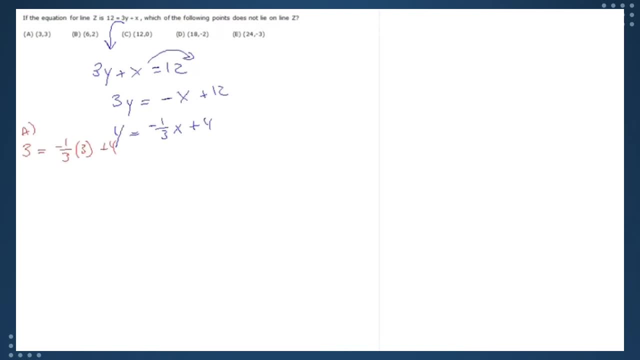 Well, if we do that math in our head, we will see that the equivalent of that will be three. So that's out. We go to B. we see that our y value is going to be two. x value is six. Doing some more mental math, we see that negative one-third times six is a negative two. 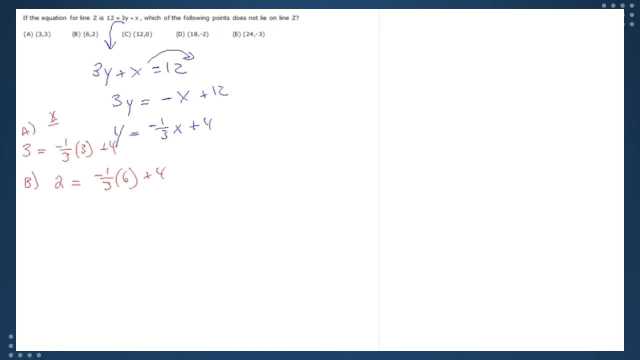 Combine that with four, we get two is equivalent to two. So that's out. Doing answer choice C. we have the y value being zero, So it's zero. Zero equal to negative one-third times 12 plus four. We see that that ends up being zero. 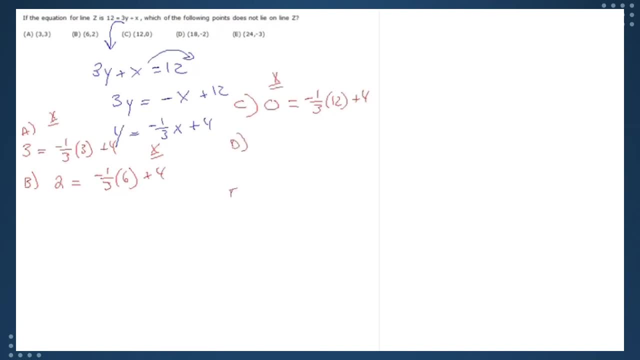 So zero does equal zero. So now the answer is going to have to be D or E. The y value we have. negative two is equal to negative one-third, So that gives us negative one-third times 18 plus four, So that gives us negative two equals negative two. 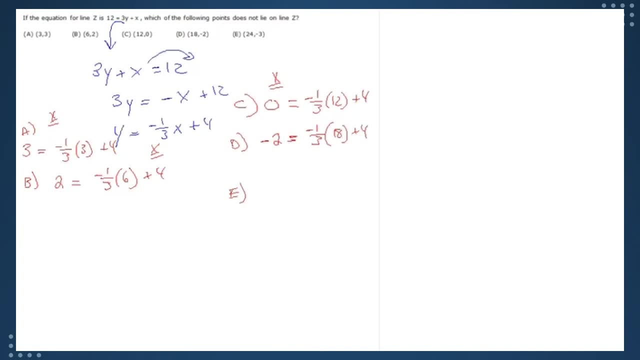 So really we have the answer being E. Now could we have started with E and moved backwards? I've heard different things about that. The answer is yes. So you know, I would let anyone kind of as they decide they want to do that. And you can do that. So you know I would let anyone kind of as they decide they want to do that And you can do that. So you know I would let anyone kind of as they decide they want to do that. 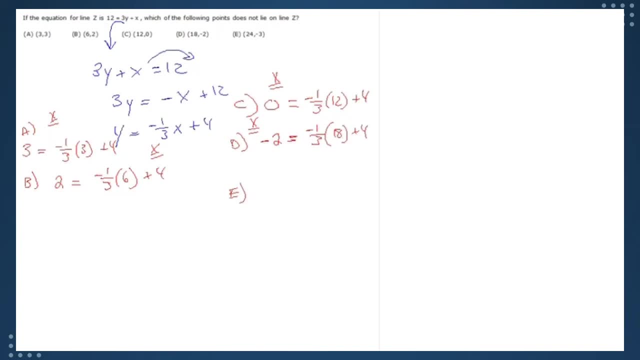 And can you leave the equation as it is? Yes, You don't necessarily have to make the standard form of the equation. I just. this is again about being systematic and doing the same thing every time. Just to prove that the third equation is good, we have negative three, being the y. 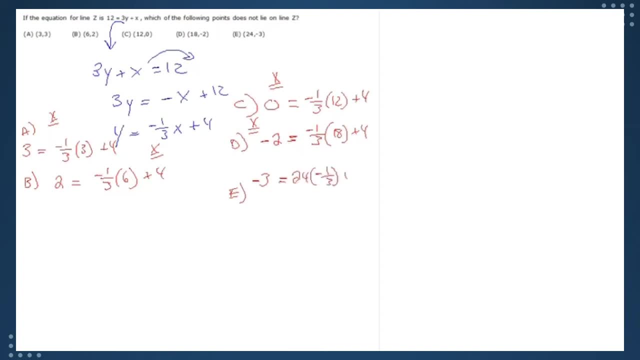 We have a 24 times negative. one-third plus four. Does negative three equal negative eight plus four? Does negative three equal negative eight plus four? No, it absolutely does not. So the correct answer is E. Next, I want to do this same idea, but not with real numbers. 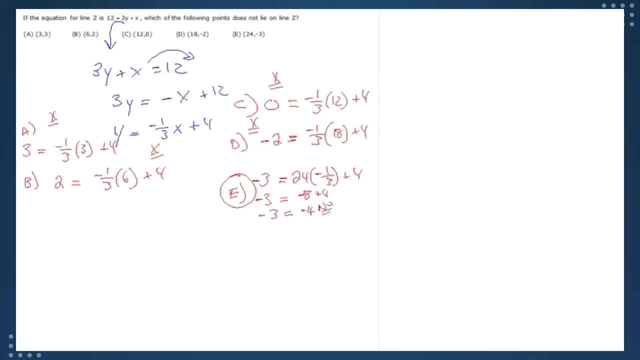 And this is going to make this idea a little bit harder, But, as you'll see, it's not that bad if you stick to your principles and do the same things over and over. So everyone, two minutes, and then we'll talk about this. 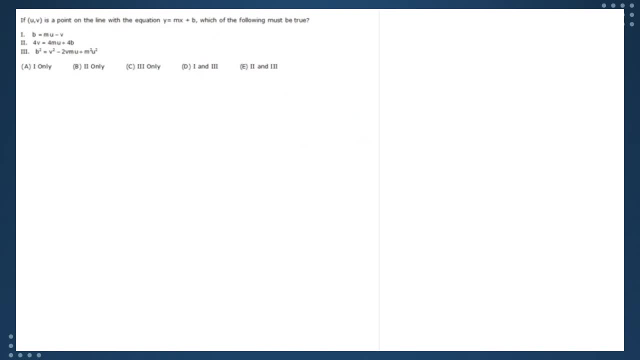 you, you, you, you, you, you. okay, this is similar to the last question. we are given that point UV is a point on the line with general equation Y equals MX plus B. so V goes in for Y, you goes in for X, and we're trying to determine which of the following must be: 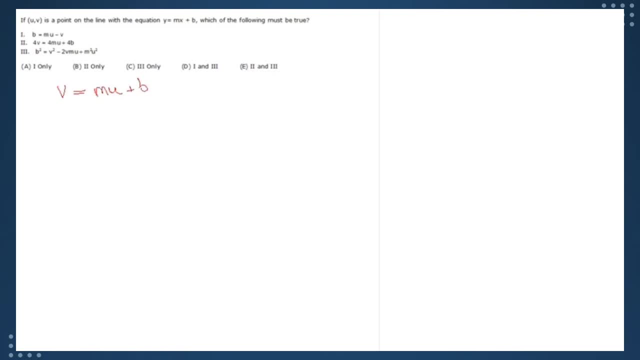 true. so the first thing is, this is really about manipulation, right? so if we were to try to make this match Roman numeral one, you have to match it for it to be true. so if we were to isolate B, we would say B equals V minus MU. now, if you look, 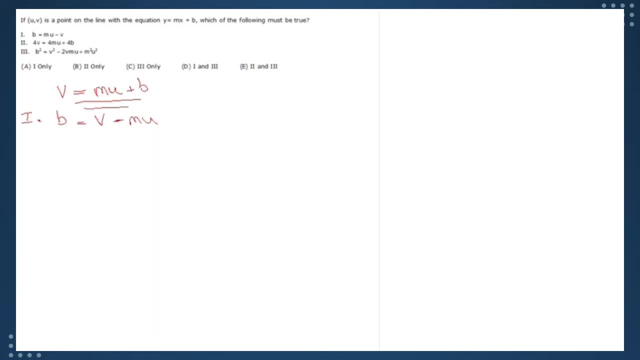 very closely. that's actually opposite the right-hand side of what you see in Roman numeral one, which is MU minus V. so that's not something that must be true. Roman numeral two: we get four V equals four M, you do, plus four B, so as you'll see, we have a four across the. 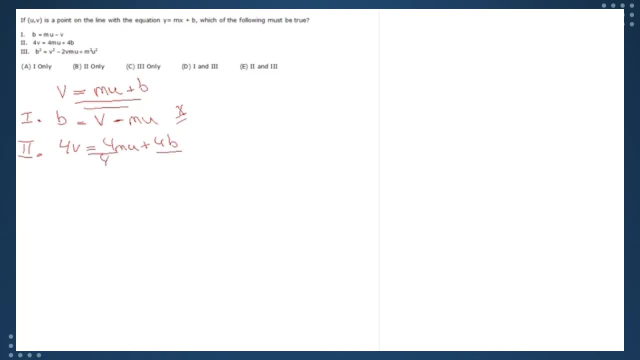 board each term. you divide by four, you get V equals MU plus B. now, if we go to our original, we see that that matches directly. so anything with a 2 in it is a good answer. so now it's just a matter of okay, is it going to be 2 and 3 or just 2? so the 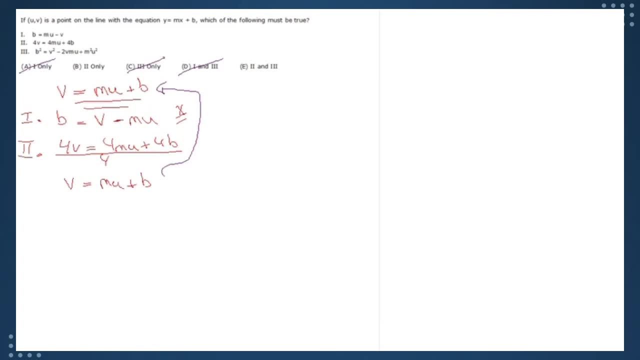 last thing we have is B squared equals B squared minus 2, V, MU plus M squared, u squared. so what I would do here is I would get the B isolated from our original equation, which is this, and actually I just apply there. nope, that is our original equation. so we would have B equals M, U minus V, excuse me, B minus M. 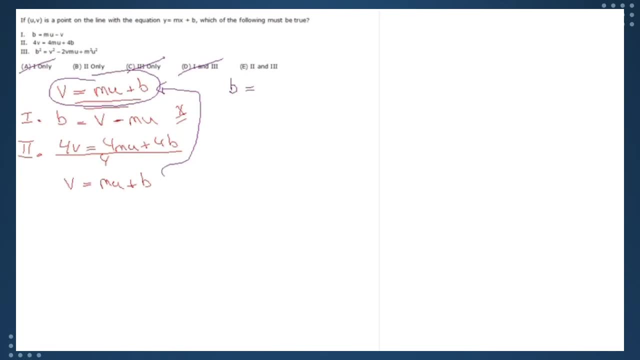 you almost got that wrong. that would have been bad, and what we're going to do is we're going to square both sides like like this, and we're going to see if they match up. now what we're doing essentially is a foil where we have E squared equals the squared minus 2 and 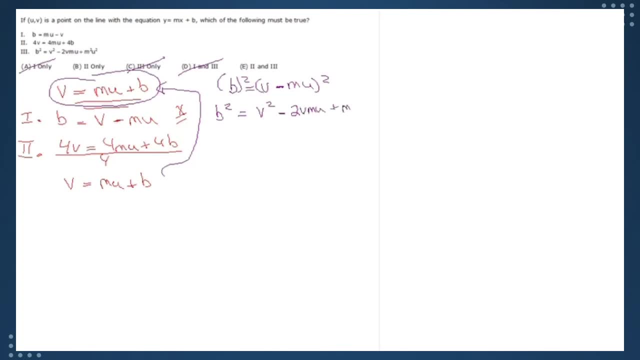 excuse me, vmu squared, u squared, and what you find it does equally. if anyone's wondering how I did that so quickly, don't forget that x minus y, all squared, which is a quadratic identity which we have a lot of in chapter 2, is x squared minus 2x, y plus y. 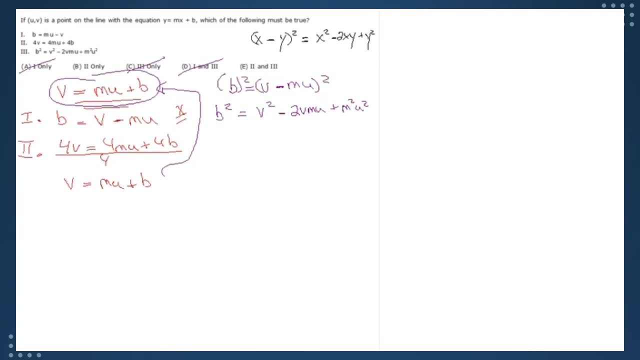 squared. so I did that kind of in my head notice: the v squared is the X, the M squared, u squared is the y squared and the minus 2 v and u is the same things: 2x, y. now I would say this is definitely on the upper echelon of difficulty, of. 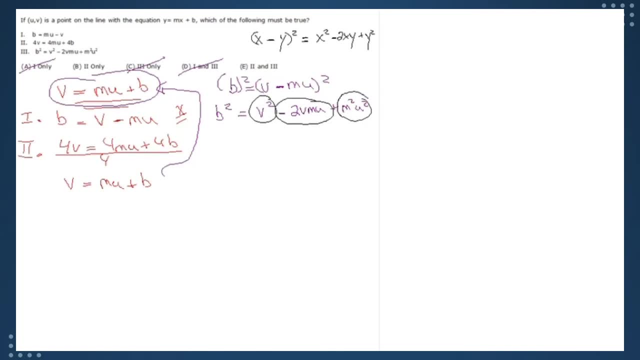 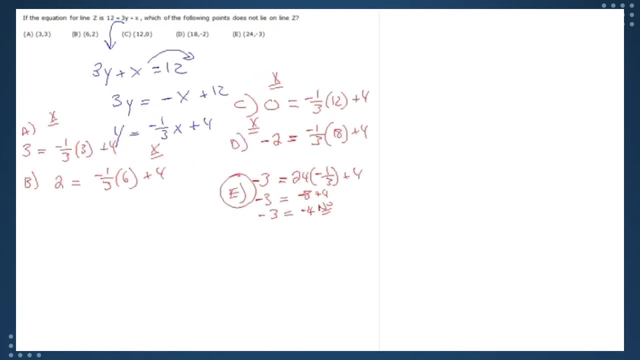 questions just because of kind of the. you know the less straightforward nature of what's happening. the last question, as you can see, although similar, you were working with real numbers, so nothing was all that. you know the less straightforward nature of what's happening. the last question, as you can see, although similar, you were working with real numbers, so nothing was all that. 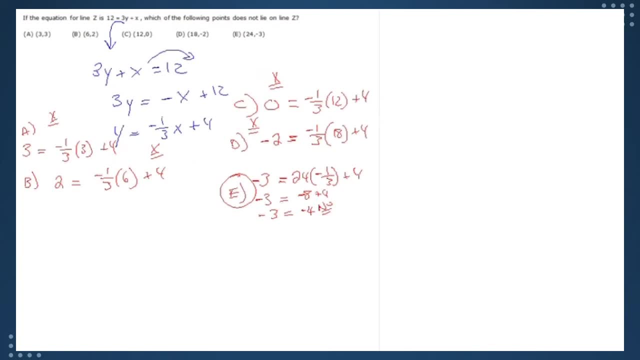 challenging and, as people had mentioned, there were many different ways people were able to get through that question. so, all in all, I think that's a very good question, something that I think everyone should be able to handle, and if you cannot, then you know. obviously this is something you want to. 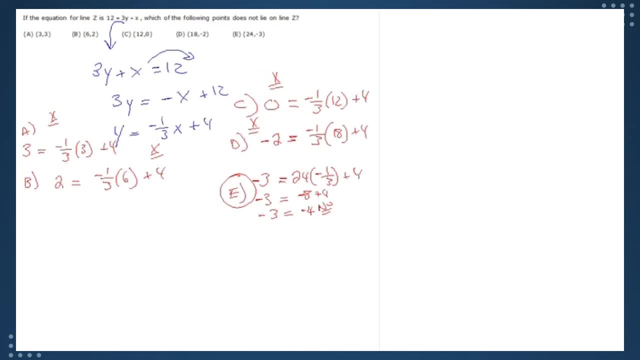 work on one quick thing I do want to do. I imagine this won't be too bad for anyone, but I do want to talk about actually developing your own equation of the line, and I want to do that here with this next question, and give everyone two minutes and I want to start to talk about. 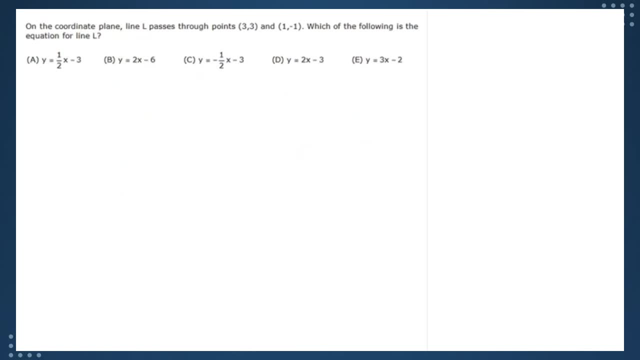 shapes in me according to point you- you- this is a bit of a talk about this with the other stuff. okay, this is a question. I also have something to add about you mauvais. I see, like you, like you, I did like that, but you build up IVS. 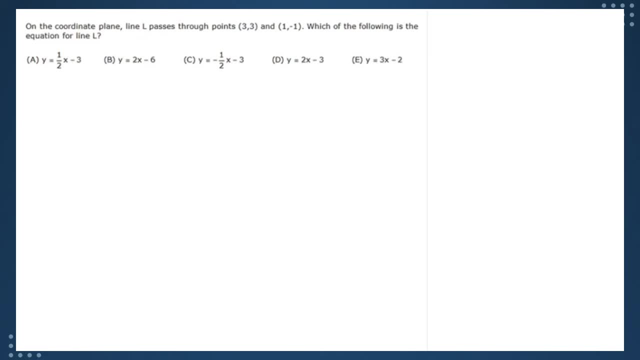 yeah, yeah, so two minutes. this question is nice and you know, cut and dry, black and white it's about: can you take a number of points and set up a equation of a line? and this is interesting to see too, because it goes to show that if you have 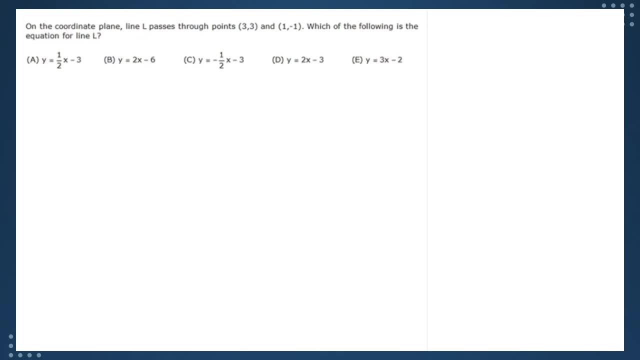 two points. you can set up an equation of a line, so for other types of questions that can be asked. you know these are good things- to know what, what you need or don't need to set up the equation of a line so you can start at any place. you. 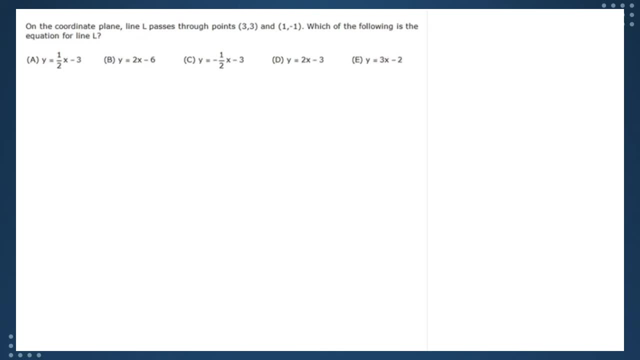 want. logically it would make sense to do the slope. so remember the equation of the line is: y equals MX plus B. so if we start off with the slope formula, the slope formula is change in Y over a, change in X Delta Y over Delta X. we see, 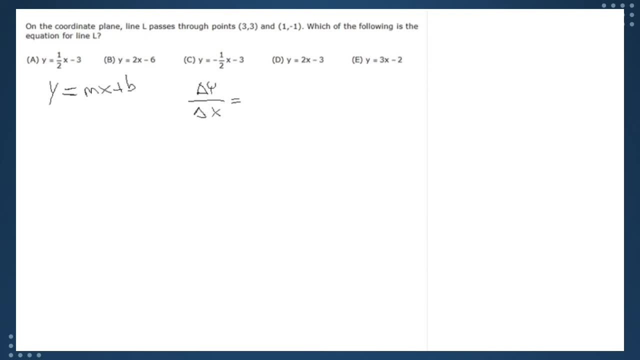 that the Y and one of the Y terms is minus one. so we can say minus one minus three. then one of the X terms is one, so one minus three. so be careful with your signs. we get a minus four on the top, a minus two on the bottom, which nets out. 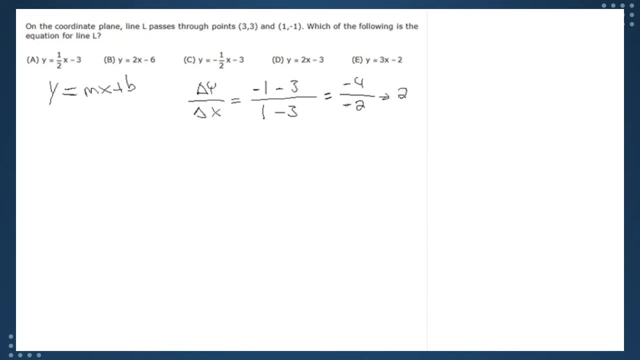 to be a positive two. so if you're running low on time, you could all intents and purposes get rid of A, C and E, because you know the slope is two. so now what you do is you set up your equation of a line and you're going to 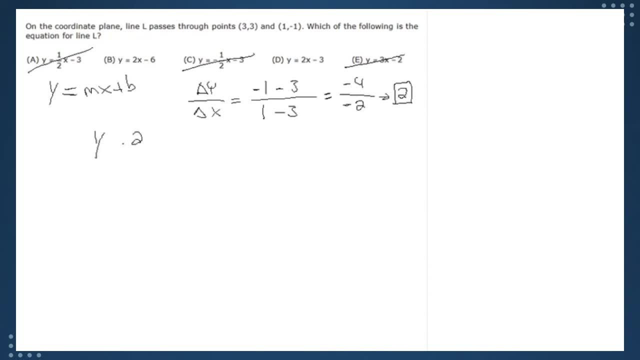 set up your equation: y equals two, X plus B, where B is the y-intercept, as we've said. then you take any set of points and plug it in. I'm going to go to a three and three. three equals two times three plus B. three equals six plus B negative. 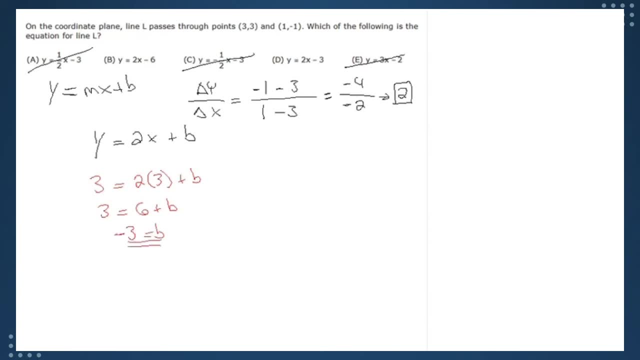 three equals B. so if the y-intercept is negative, three equation of the line is: y equals two X minus B. So I do hope that anyone taking the test sees something like that. it would be great, because this is one of those things where you know how to do it you. 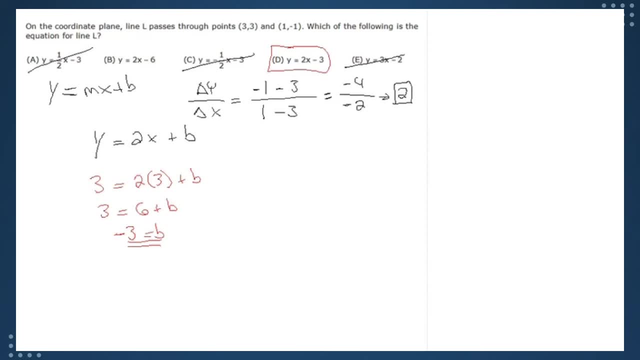 plug in, you get your line, you move on, and to me, that's one of the better ways to be able to deal with questions on the test, because it allows us to be incredibly, incredibly systematic. I want to do one last question. this is definitely going to be a good one. 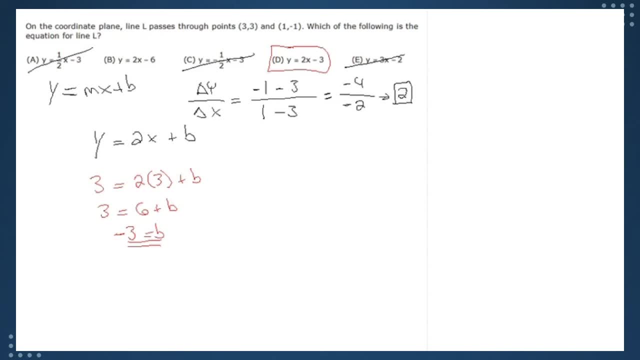 It's going to be as hard as what we've done today. it's in a very challenging nature- test us on shapes in the coordinate plan. so we'll give everyone a couple minutes then we'll spend the necessary time on this. Thank you, you all. right, since we don't have a ton of time, we will begin kind of sketching this out now. remember it's. 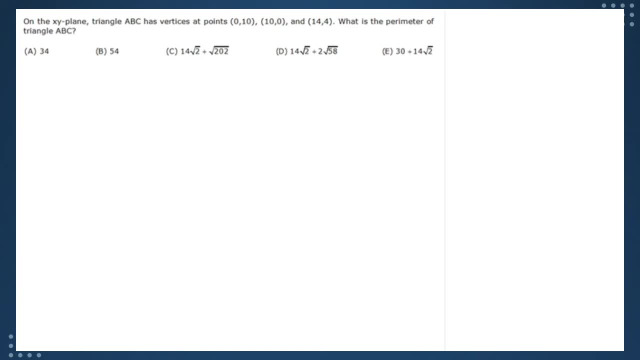 possible that you'll have, you know, the use of graphing paper and stuff like that, graphing lines, which is definitely something that will help as you do a problem like this. I'm going to make kind of my own graph like thing here, my X and Y axis, rather so there's your zero, there's your X and your Y axis, and 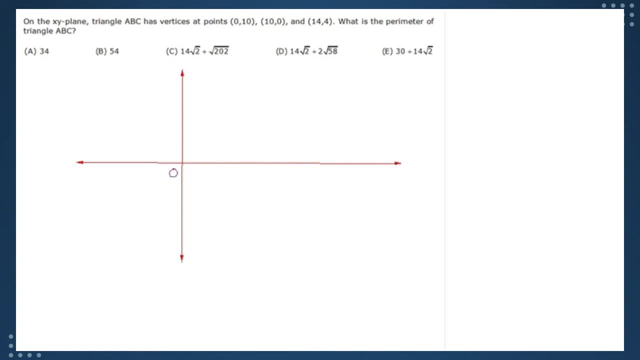 so we have a point zero, ten, so zero. move up ten. so we're going to just kind of ballpark this over here and we have ten, zero- remember this is not done to scale, so don't think it is- and then 14.4, so we'll say that's roughly here. now what? 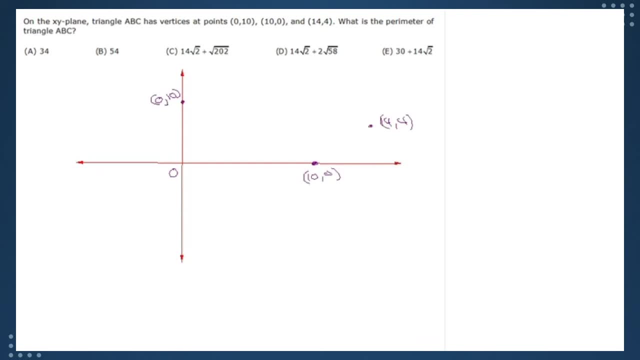 everyone's going to do is we're going to do, is we're going to do a little bit of a rough sketch here, and we're going to do a little bit of a rough sketch here and we're going to do a little bit of a notice that this is an awkward shape. now, if you've read our geometry chapter, 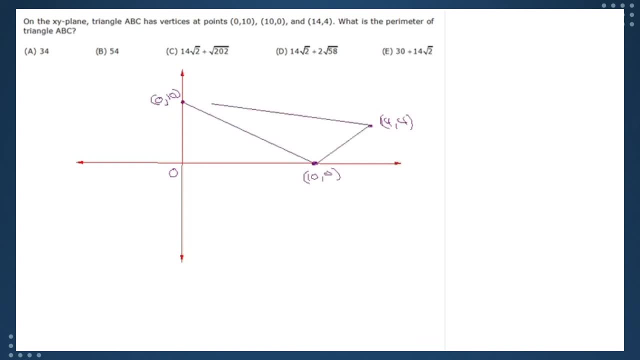 we teach about how to potentially deal with awkward shapes, but in this particular instance, there's no way, no how, that we are going to be able to get the perimeter of this by just looking at the lines. and if they ask for area, this is another thing that you would be able to do for it. but strategically, what's? 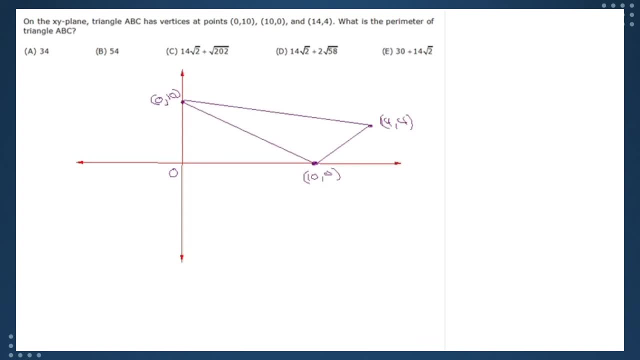 really cool here is we can actually create a bunch of right triangles from making really a rectangle around this triangle, pointing all the points, and I'll put a little right triangle sign so you can see the right triangles. so what we did, what we're going to do, is we're 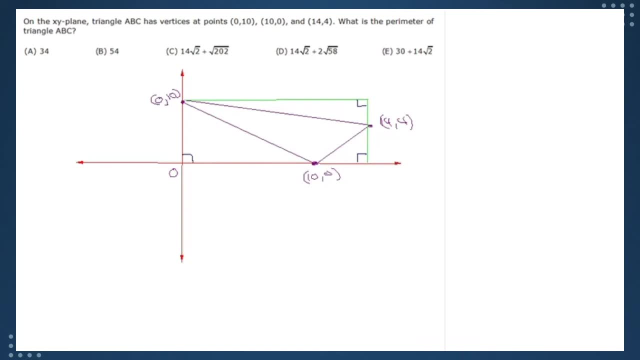 basically going to use the Pythagorean theorem here to come up with the size of each one of these triangles. so, for instance- let's start with something easy- we have a ten, we have a ten, okay. well, the Pythagorean theorem says that 10 squared plus 10 squared equals C. 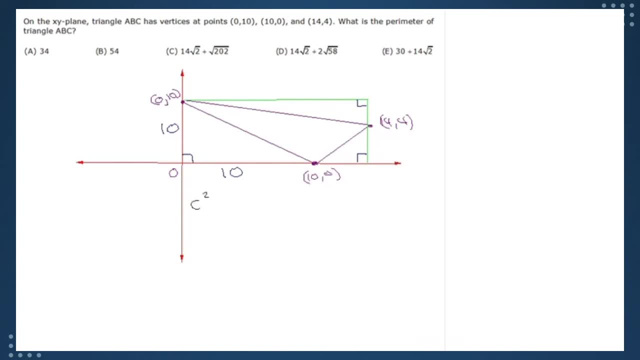 squared. so basically, C squared equals 200. C is the square root of 200, which, as we know, is 10 root 2. so anything with a root 2 in it, you can pretty much already say that's going to be a possible answer. eliminating A and B. now we can go over to the smaller triangle here. 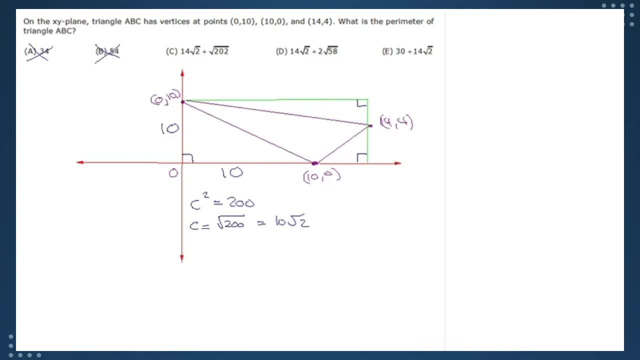 and we can say: all right, well, we know that this line has to be 4 because we're going from 10 to 14.. And we know actually that this line has to be 4 because this point here on the far right is 14, 4.. 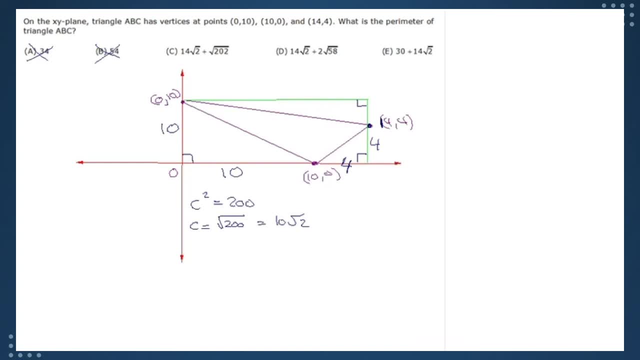 So if we do strategic a diagram theorem again, we're going to get C squared equals 32 because, remember, we're talking about 4 squared plus 4 squared, So 16 plus 16 is 32.. Square root everything and we end up with C being 4 root 2.. 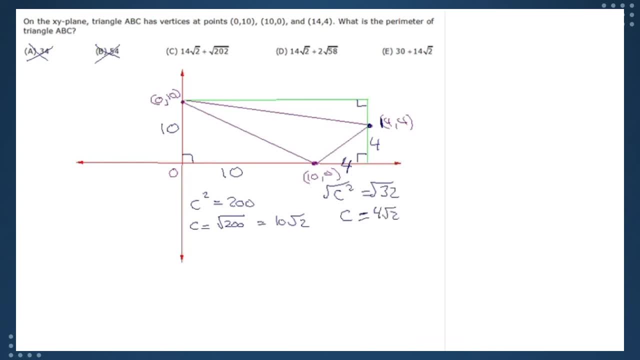 So if we add these together, we see that part of our perimeter is already 14 root 2. So we can now- well, actually we can't eliminate anything, unfortunately. So now we go to the last component and we see that the big triangle- 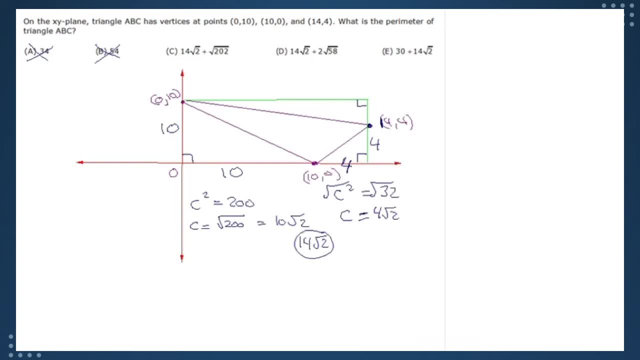 this has a height of- well, it's going from 4 up to 10.. So the height of that is 6.. And again, remember I told you it wasn't drawing a scale And this here is going to be 10.. 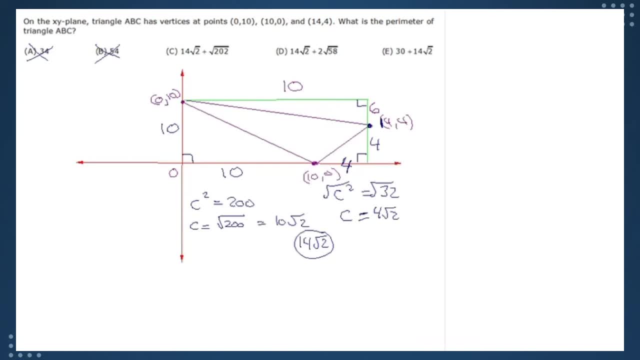 So we have 10 squared plus 6 squared equals C squared, So we have C. Let me just make sure that's right. You know what I'm making a short small mistake there. That's not 10.. That's 14.. 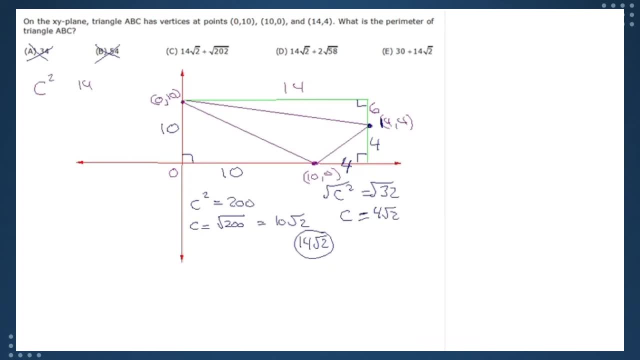 So we have C squared equals 14 squared plus 6 squared. So yeah, this number is getting a little large. I get that 14 times 14 is 196.. Of course, 6 squared is 36.. So if we add these together, we get C squared equals 232.. 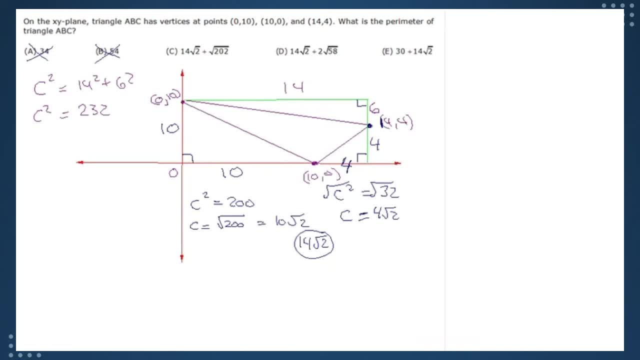 So, strategically, at this point, you can actually finish this, this question, without completing out this to the bitter end, because what we know is we're looking for this final value here And I can tell you that, since we already have 14 root 2,. 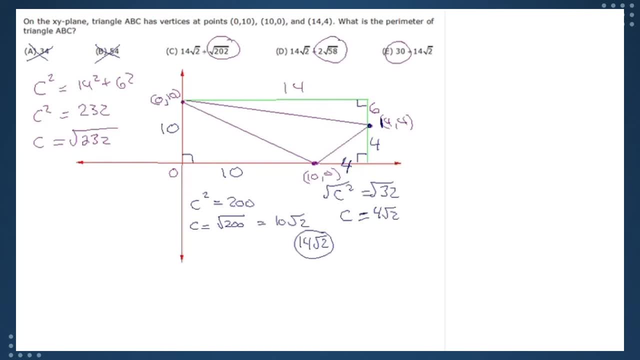 about what's the final value in the answer choice. Well, look, square root of 232 is not the square root of 202.. The square root of 232 is not 30. So the only answer that's logical here is 2.. 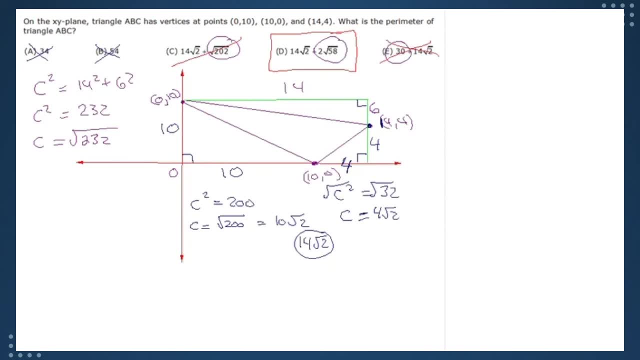 And the answer here is root 58.. And this is something I want everyone to take into account. Sometimes you don't have to go to the bitter end in your answer choices, so the answer here is D. This is a tough one. I'm glad we ended on this one. 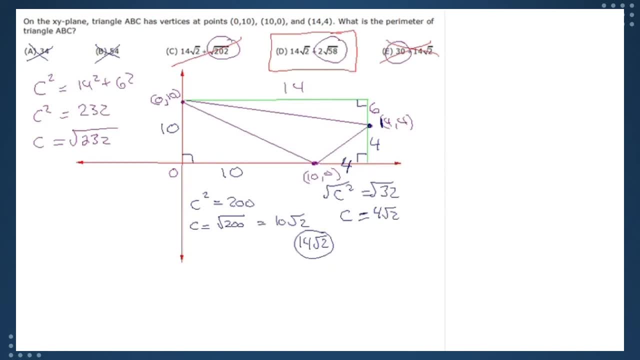 You know, like always, hopefully you can take away some things that we did here today and start to use them on your own, As always, you know. thank you. I want to thank everyone for coming. If you have any questions or concerns, feel free to reach out to me.